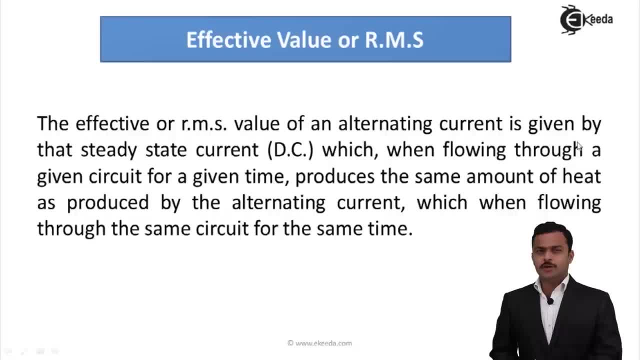 Hi, friends, in this video we are going to see the most important parameter of AC voltage, waveform, and that is RMS or effective value. Let us see the definition of it. The effective or RMS value of an alternating quantity is given by that steady current which, when flowing through a given circuit for a given time, produces the same amount of heat as produced by the alternating current which, when flowing through the same circuit for the same time. 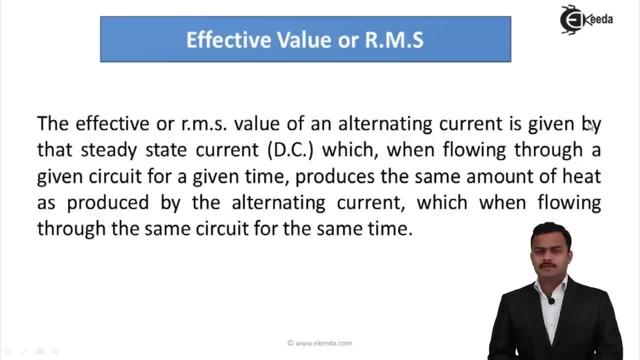 Meaning. suppose I perform an experiment where I connect a DC supply to a lamp And I will measure a power by passing a DC current for some amount of time. Now, instead of a DC I will replace AC and I will check the same effect for same amount of time. 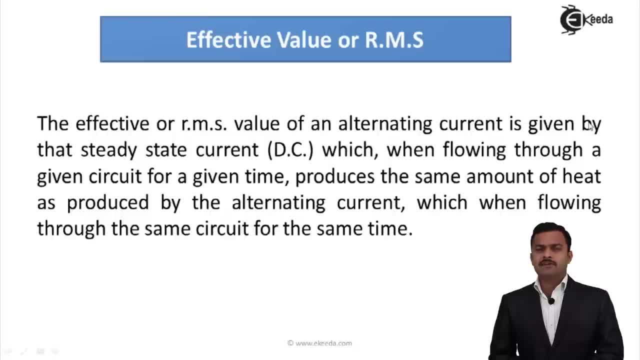 The moment, I will get the same effect: that value of AC I noted down, which is nothing but a RMS value. So in short, I can say RMS value of AC quantity is nothing but its DC equivalent Meaning. if I replace the RMS value of AC with the same amount of DC, I will get the same effect. 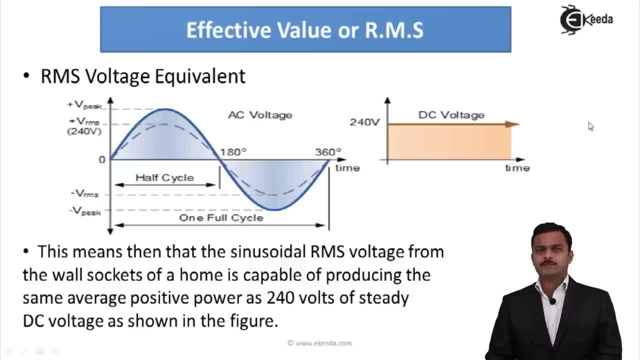 So let us move to the next point. The next point is: I will elaborate the same concept with an example. So what I have over here? I have an AC supply given by the socket And I will measure the effect. Suppose it is giving a 240 volt AC. 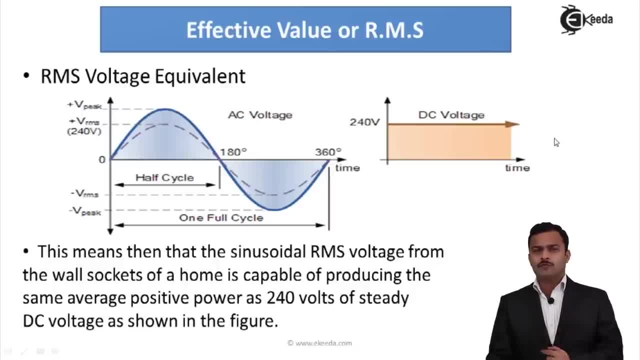 240 volt AC is doing the same amount of work as if 240 volt DC. So this particular example will clear the idea of RMS. So what is the advantage of RMS value Everywhere AC is denoted by its RMS value? Because RMS value of AC is nothing but a useful component of AC voltage or AC current. 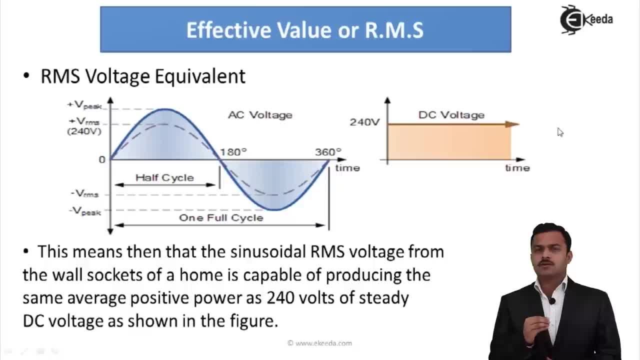 Which is responsible for production of RMS, Production of actual power, or responsible for doing a work. done So everywhere. whenever we see a voltage, that is always a RMS value. Just take an example: whenever we have a domestic household supply that is single phase 230 volt AC 50 hertz. 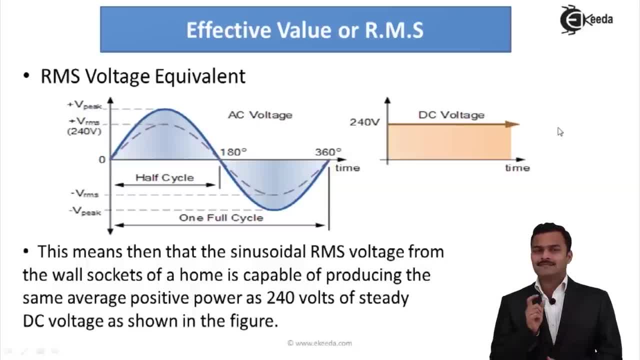 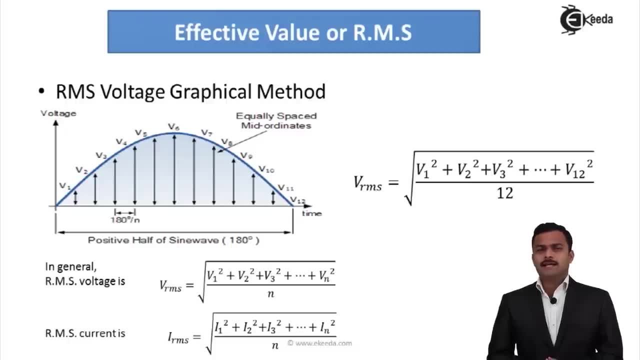 So this 230 volt is nothing but a RMS value of AC supply. Now effective value can be calculated by two ways. One is a graphical and second is a analytical way. So let us say a graphical method. So in graphical method I have considered only a half cycle. 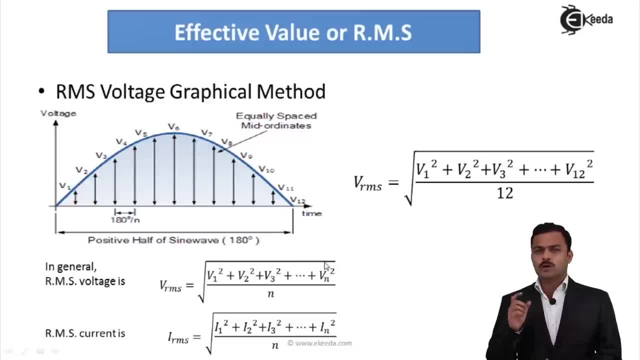 So its RMS is nothing but a root mean, square. So what we have to do, We have to take a mean of square of every instantaneous values And then we have to take the square root of it. So what I have done? only half wave, I have considered: 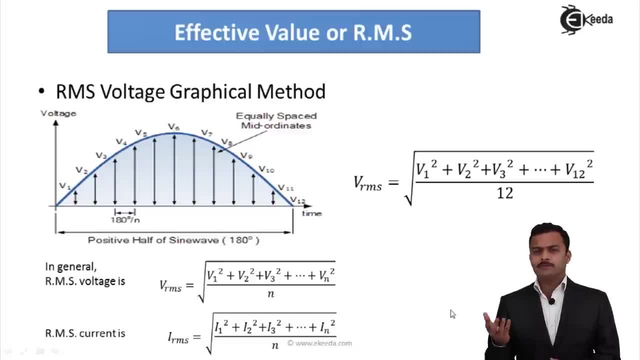 Only half cycle I have considered, So same effect can be true for a full cycle. So in half cycle. I have considered this 12 instants. So this 12 instants is giving you 12 instantaneous values of voltages. 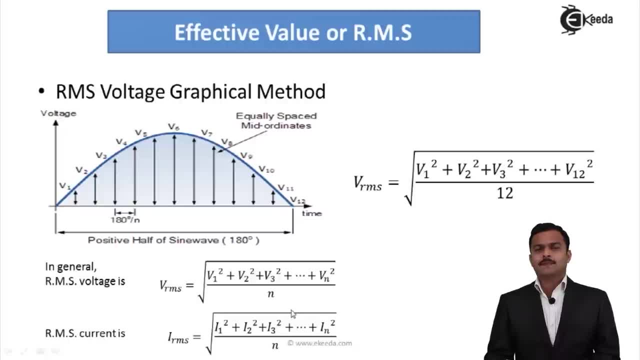 V1, V2, V3, like that. So as per the definition, it is a root of mean of Square of instantaneous values. So that will give you VRMS equal to root of V1 square plus V2 square plus V3 square, like that. 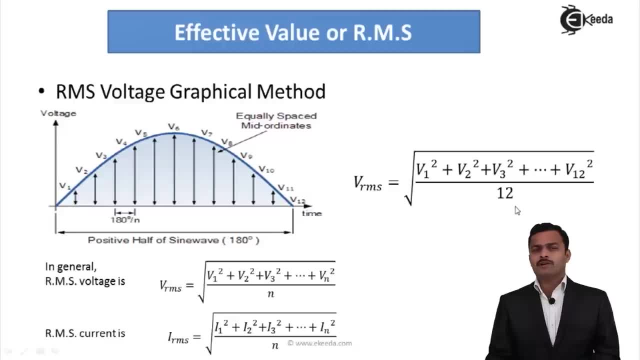 Till V12 square divided by 12, because I have considered 12 values In general. if I have n number of values, I will get RMS voltage as VRMS equal to root of V1 square plus V2 square. like that, Till Vn square divided by n. 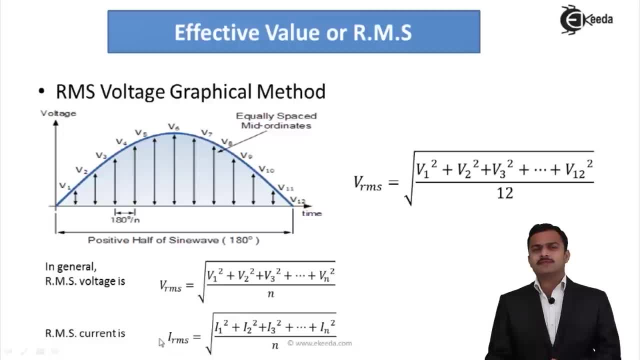 For a current. if I replace V by I, I will get IRMS as root of I1 square plus I2 square plus I3, square up to IN square divided by n. So in a graphical way, what we do a waveform, we split it into number of instances. 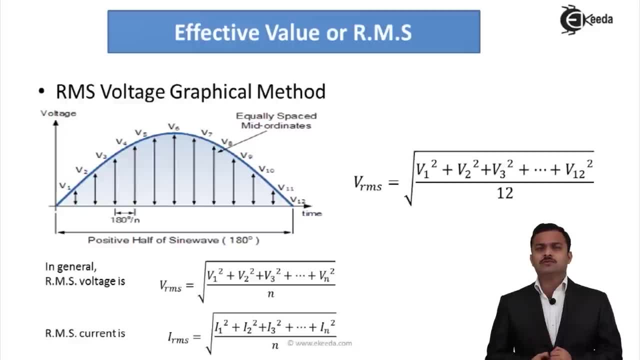 And for every instant we get the instantaneous value, Square it. Likewise, we take addition of all the squaring of all the instantaneous values Divided by number of instances we are considered, And then ultimately, we take a root, We will get a RMS value by a graphical method. 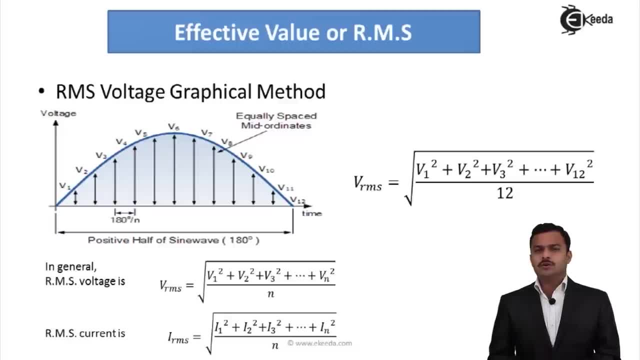 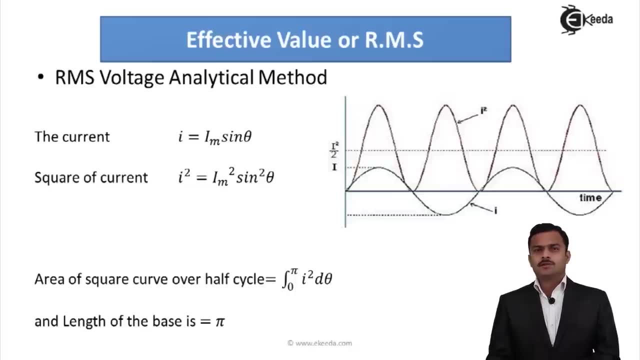 Suppose I want to find out RMS value by another technique, which is analytical method. See how we are going to do that. So the current is given by I, equal to IM sine theta, a standard AC current waveform. Then let us square it. 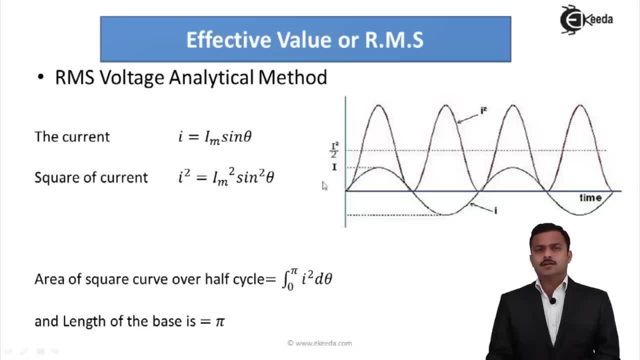 So I get I square equal to IM square sine square theta. So in this figure I have shown the IM sine theta like this, And squaring of it will be like this. So what we are doing, We are considering the area under this curve which is nothing but a integral 0 to pi: I square d theta. 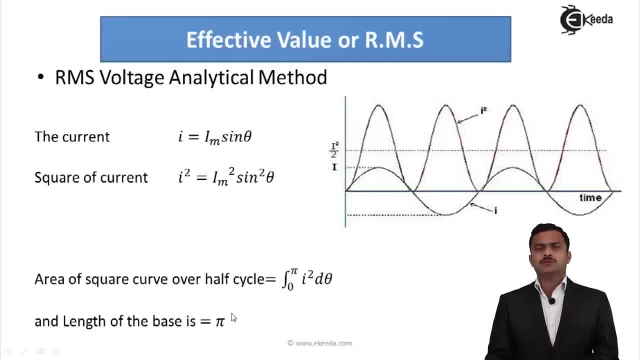 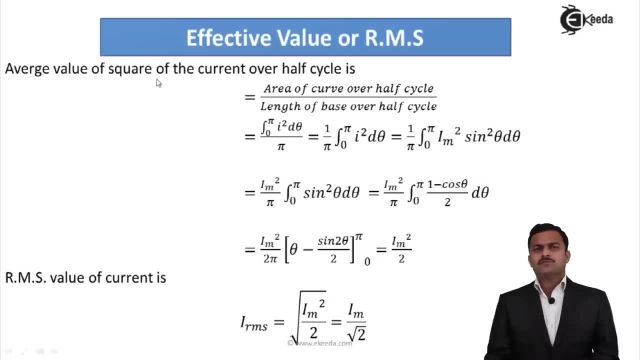 And length of this is nothing but pi because we are just considering half cycle. So if I solve further What I will get? Average value of square of the current over half cycle is given by area of curve over half cycle divided by length of a curve for half cycle. 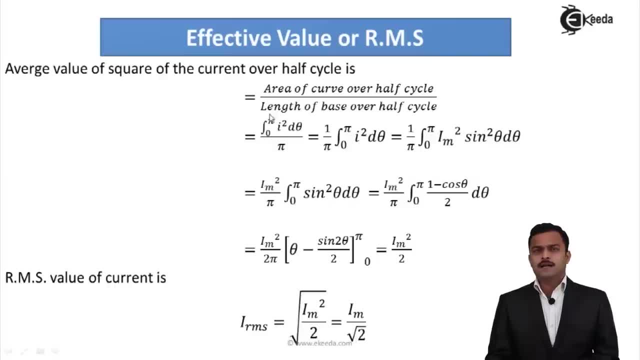 So it gives me integral 0 to pi. I square d theta divided by length is pi, So that is ultimately 1 over pi. I can take it out 0 to pi. I square d theta Then 1 over pi. 0 to pi is a limit for integral. 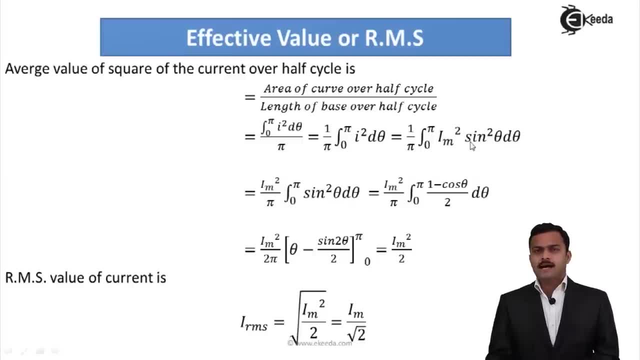 I we know, is IM sine theta And squaring is IM square sine square. theta d theta We know sine square. theta is given by 1 minus cos 2, theta divided by 2.. So I have replaced that constant I will take out of integration. 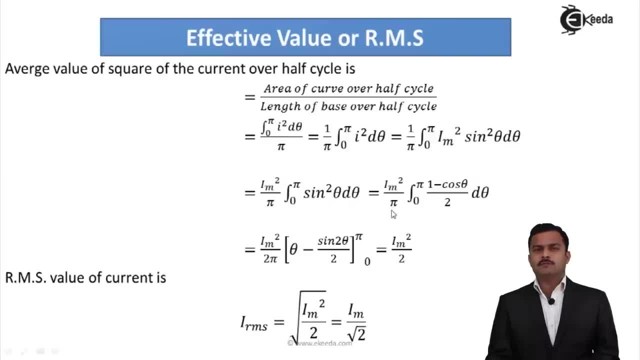 So I will get this expression: IM square divided by pi integral exist from 0 to pi 1 minus cos 2. theta divided by 2 into d: theta Integral of 1 is theta If I take a 1 by 2 common.